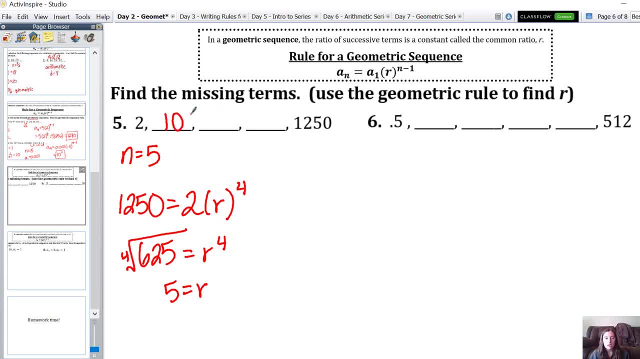 by five each time. So two times five is ten, Ten times five is fifty. Fifty times five is two hundred and fifty. And let's make sure, two fifty times five is in fact 1250.. So that means we got this correct Number six. we're starting with 0.5, ending with 512.. Here we have one, two. 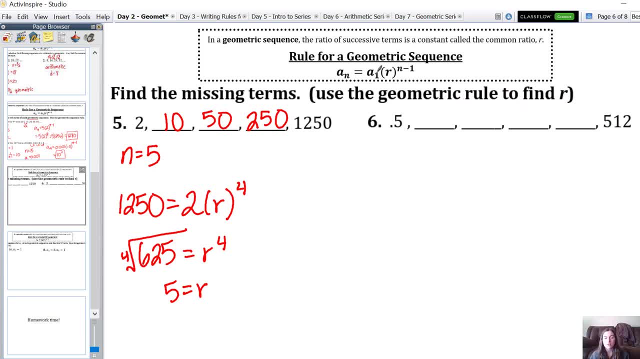 three, four, five, Six numbers. We have six different terms, So n is six. The last term that I know about is 512, equal to the first term that I know about, 0.5 times r to the six minus one, which is five. So 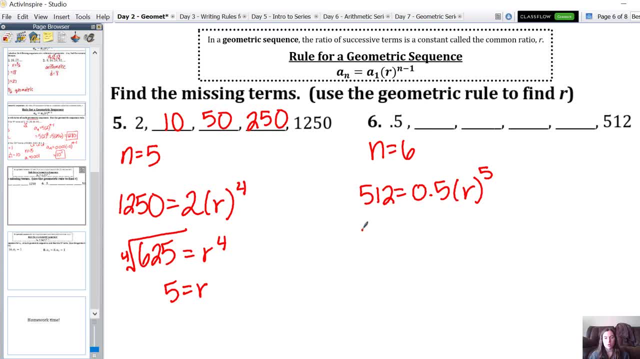 now we need 512 divided by 0.5, which is 1024.. That's equal to r to the fifth. Now we're going to take the fifth root of both sides And our value of r here is four. That means each time we're multiplying by four, So 0.5 times four. 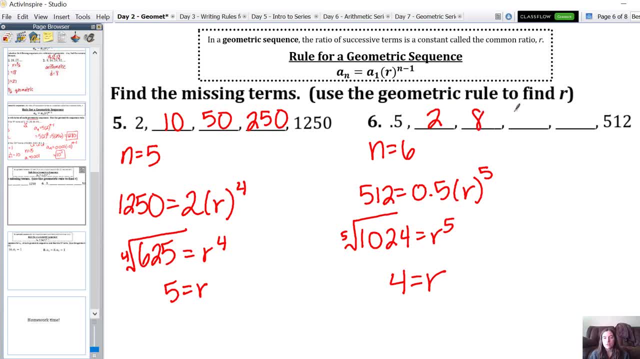 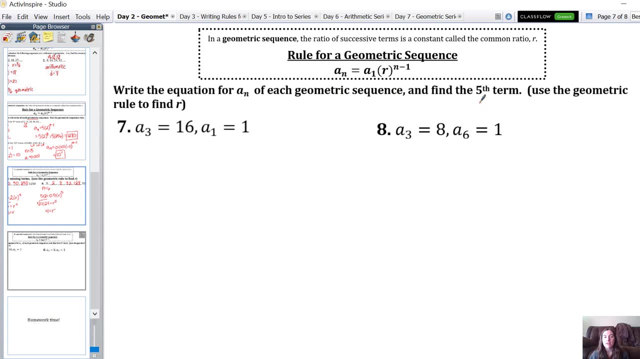 is two. Two times four is eight. Eight times four is 32.. 32 times four is 128. And 128 times four is 512.. Now we need to write an equation for a sub n of each geometric sequence and then find: 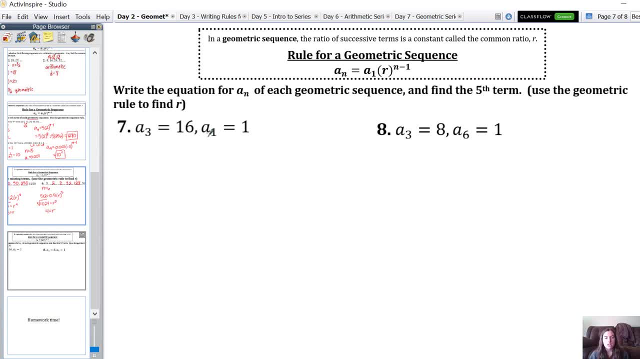 the fifth term. a sub three is 16.. And a sub one is one. First I need to figure out what r is, And then we will figure out our equation and our fifth term, The last term that I know about. is this a sub three? 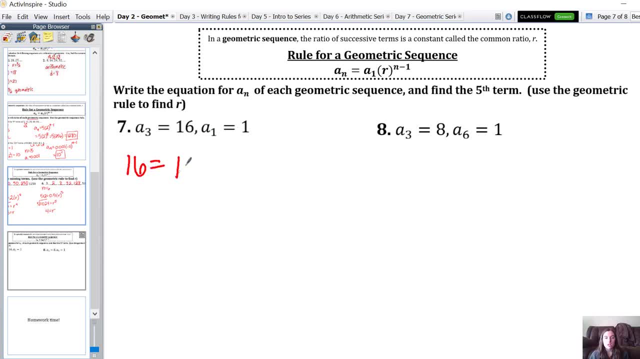 I'm going to use that number equal to my first term, which is one times r to the power of. And then we have one, two, three to get from a sub one to a sub three, And three minus one is two. So now we have 16 equal to r sub three. 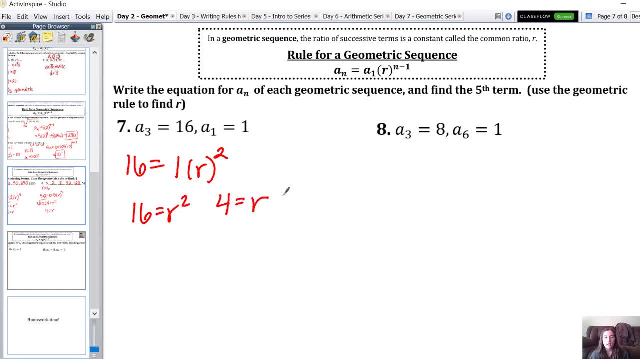 squared, which means our value of r is 4.. So our equation in general would be: a sub n equals 1 times 4 to the n minus 1, which you could also just write as 4 to the n minus 1, because 1 times. 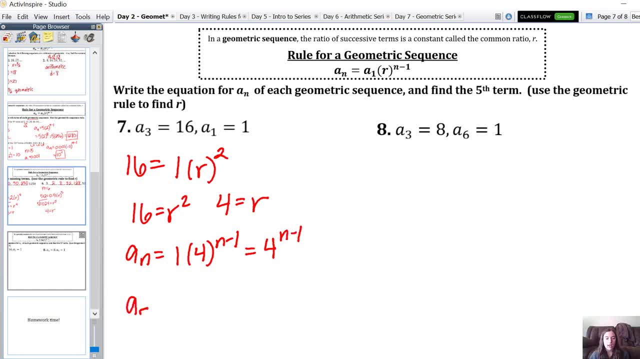 that wouldn't change it. So now for a sub 5, we need 4 to the power of 5 minus 1, which is 4 to the fourth, which is 256.. In number 8, we have a sub 3 and a sub 6.. I don't have a sub 1, so the 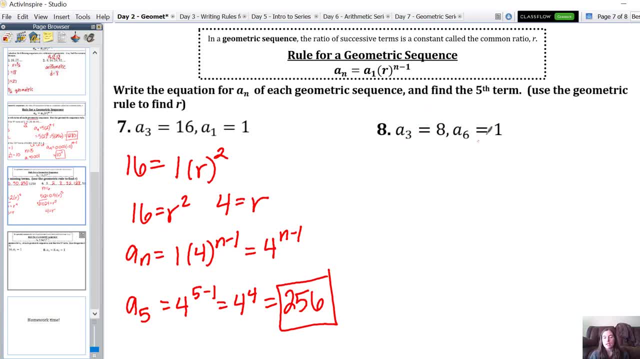 first term that I know about is this a sub 3.. The last term is a sub 6.. So let's figure out what a is To get from a sub 3 to a sub 6, we have a sub 3,, sub 4,, sub 5, and sub 6.. 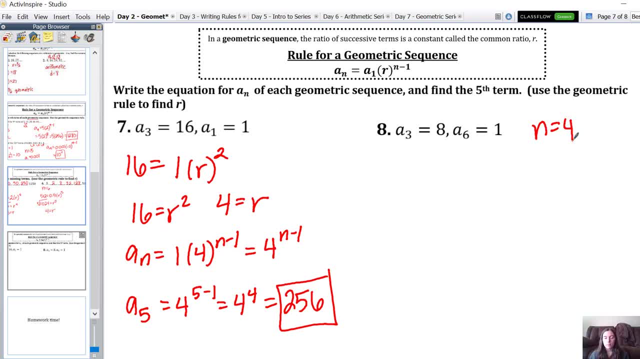 So our value of n here is 4.. The last term that we know about a sub 6, is 1.. The first term that we know about is 8 times r to the power of 4 minus 1, which is 3.. Dividing by 8, we just have 1 over. 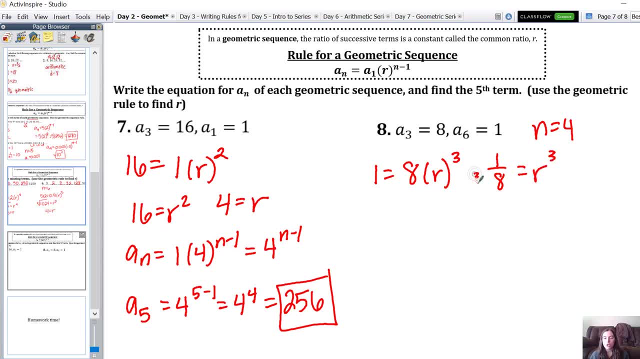 8 equal to r to the third. Now we need the cubed root of both sides. The cubed root of 1 over 8 is 1 half. So r is equal to 1 half. So our general equation would be: a sub n equals. now we don't know- a sub 1.. So to find a sub 1, I'm going to work. 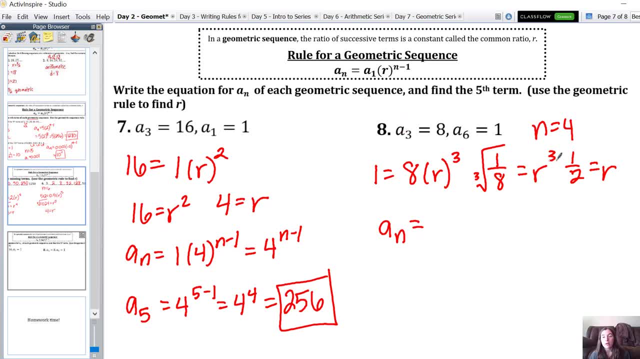 backwards from a sub 3. Since to go forward, I would be dividing by 2. So to go backward, I'm going to multiply by 2.. So a sub 3 times 2.. 8 times 2 is 16.. 16 times 2 is 32.. That means my 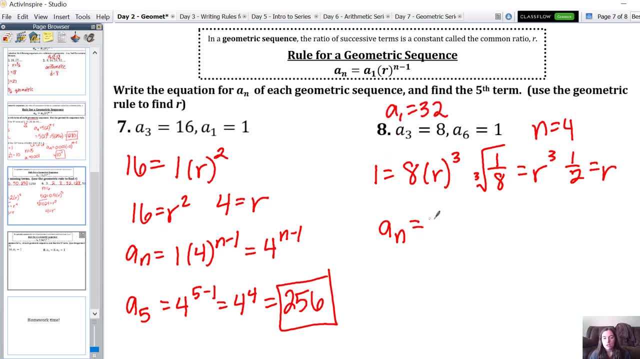 a sub 1 is 32.. So now I have 32 times 1 half to the n minus 1.. For a sub 5, I'm going to use 32 times 1 half to the 5 minus 1, which is 4.. 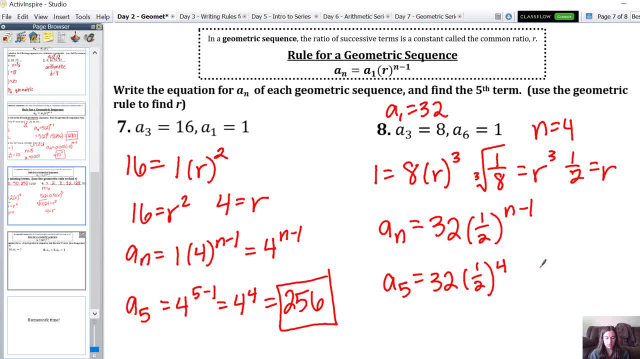 And I can put that in my calculator: 32 times 1, half to the power of 4, which is 2.. Or you could have also worked backwards from a sub 6 and just multiplied by 2, with the same idea as what we did from a sub 1.. Subtitles by the Amaraorg community.